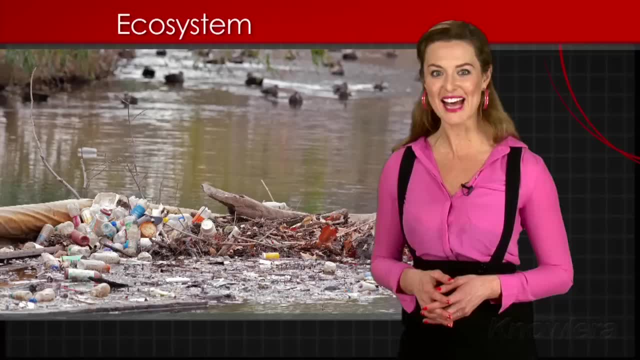 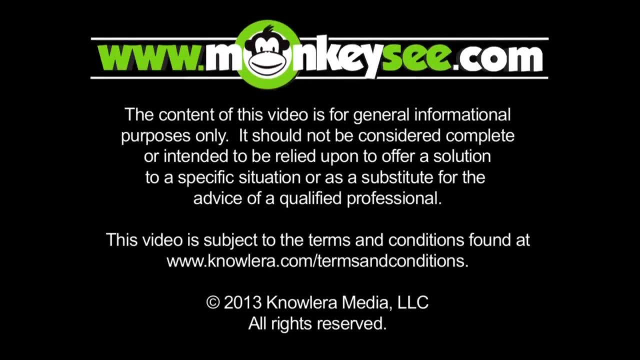 ecosystems and continually work to discover new ways to protect these precious organisms and environments. For thousands of how-to and advice videos on any topic, visit monkeyseacom. 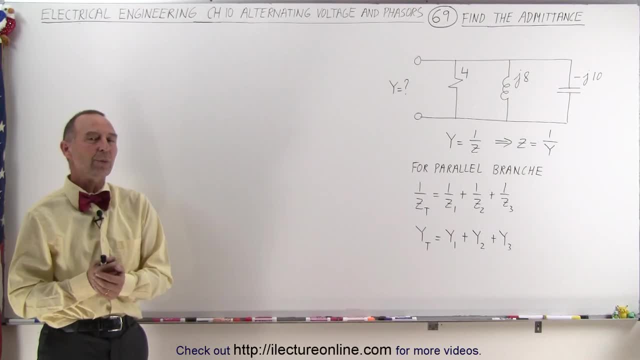 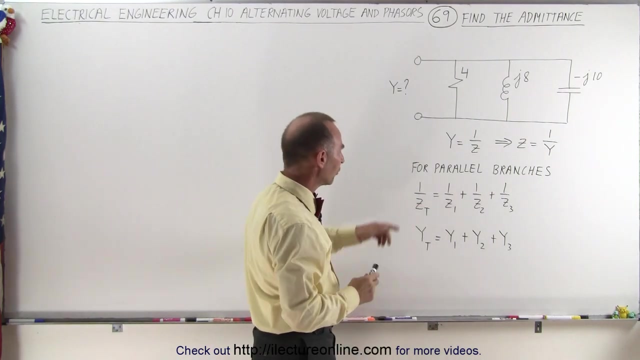 Welcome to Electron Line. When you're dealing with AC parallel circuits then you find that trying to find the impedance of that circuit can be quite challenging because we have to use the equation. Of course I'm missing an S right here, but you have to use the equation that 1 over the 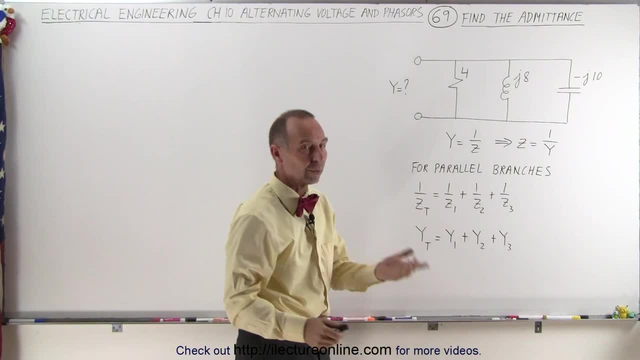 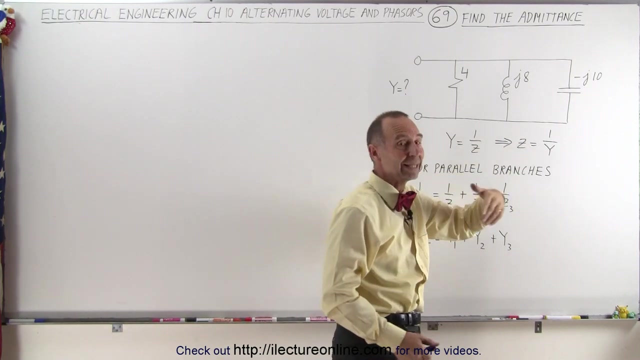 total impedance is equal to 1 over Z1 plus 1 over Z2 plus 1 over Z3 and so forth. So it might be easier to use admittance. We know that the admittance is equal to the inverse of the impedance, so that if you want to find the impedance, you can first find admittance and then simply take. 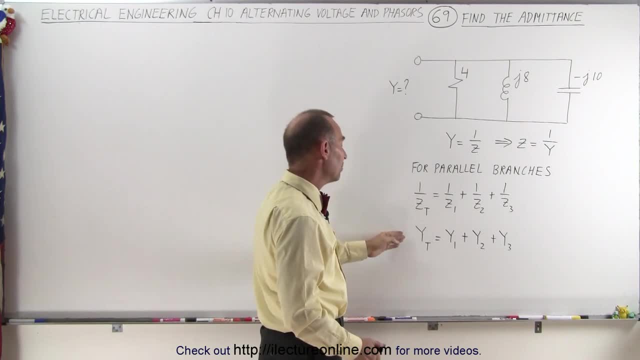 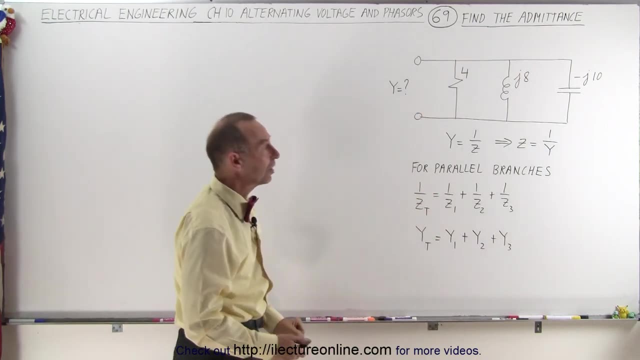 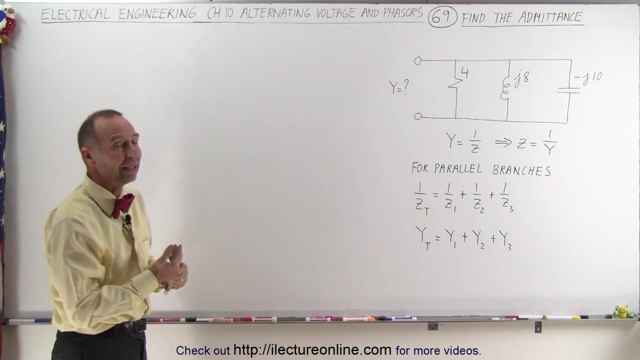 the inverse, because for parallel branches the admittance, the total admittance, is simply equal to the sum of the individual admittances of each of the components in a parallel circuit. So let's go ahead and use that technique to see how to find first the admittance of the circuit and then in the 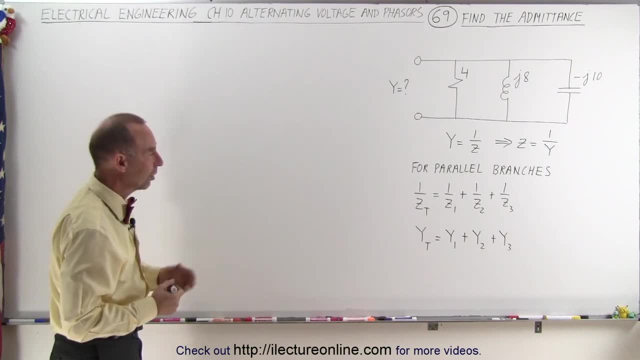 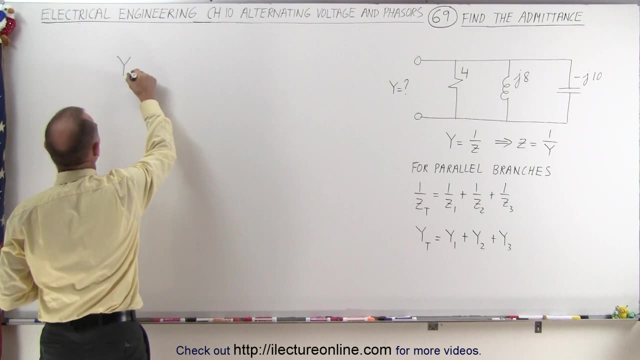 end how to find the admittance of the circuit, How easy it is then to find the impedance of that circuit utilizing this concept right here. So first we're going to find the total admittance. So admittance total is equal to admittance.